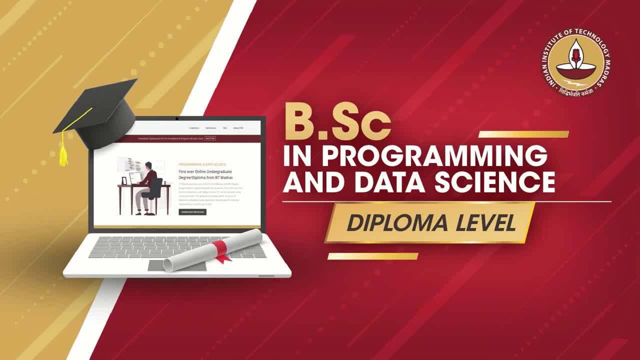 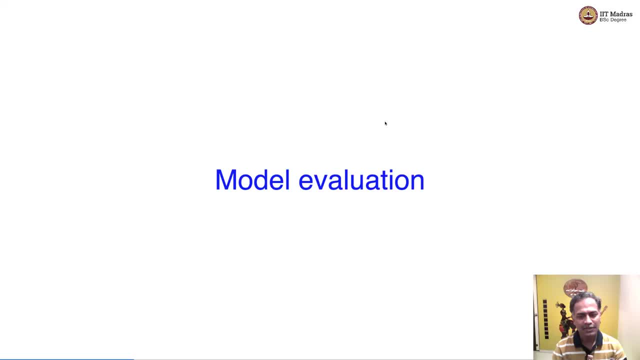 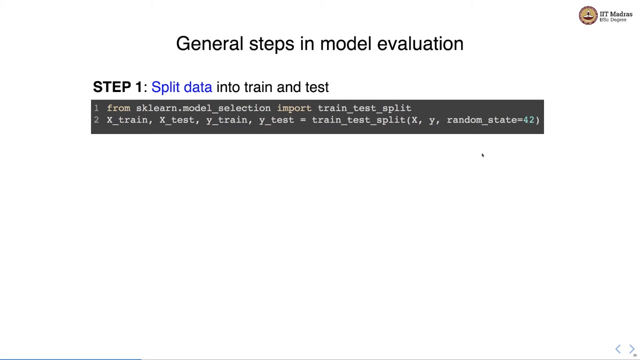 Namaste, welcome to the next video of machine learning practice course. In this video we will discuss how to evaluate linear regression models in sklearn. Let's look at general steps in model evaluation. We first split the data into training and test. For that we use train underscore, test underscore split class from sklearn dot model. 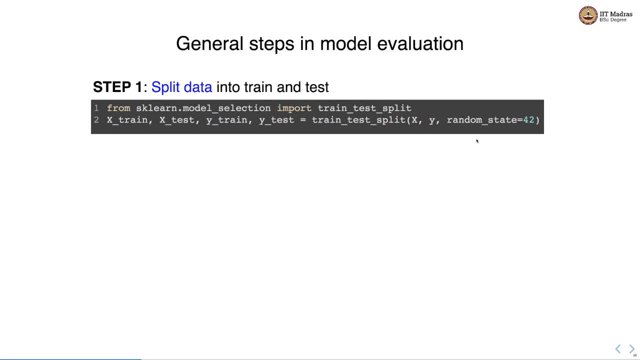 selection module: Train underscore, test underscore split takes the feature matrix X and label vector Y or it could also be label matrix in case of multi output regression. It returns the train feature matrix, test feature matrix, train labels and test labels. We fit the linear regression estimator on the training set. We calculate training error. 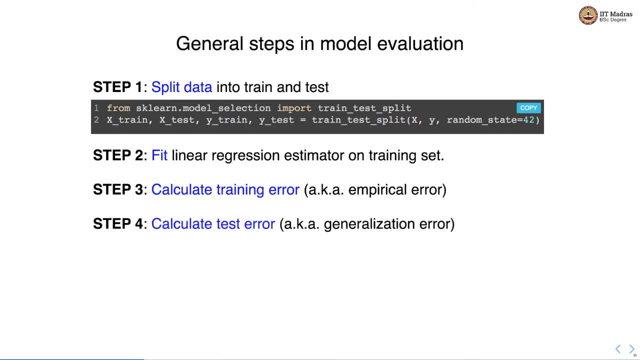 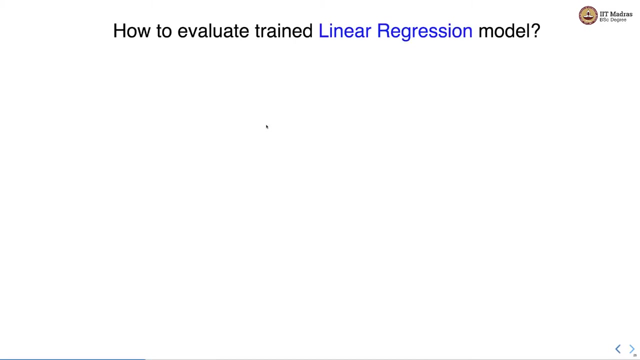 which is also called as empirical error, and finally we calculate test error, which is called as general error. Then we compare training and test error to understand whether our model is right fit or whether it is underfitting or overfitting. So let's study how to evaluate trained linear regression model in sklearn. 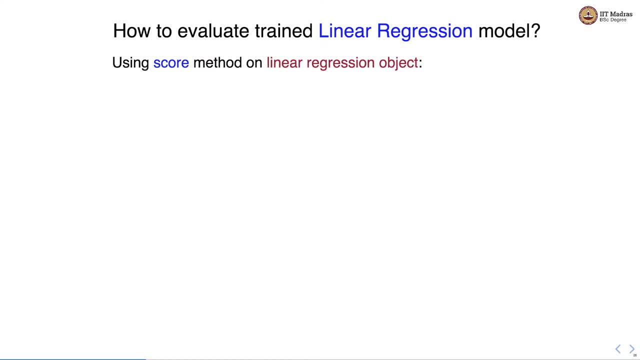 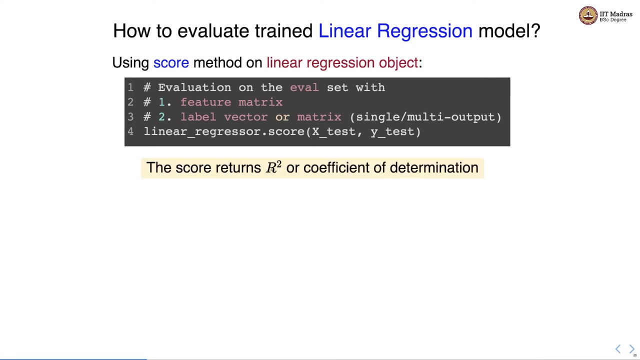 sklearn provides score method on estimator objects. We are going to use this score method for evaluating the trained linear regression model. So what we do is we call the score method on the regression estimator, We supply the feature matrix and a label vector or matrix of the test set and the score method returns. 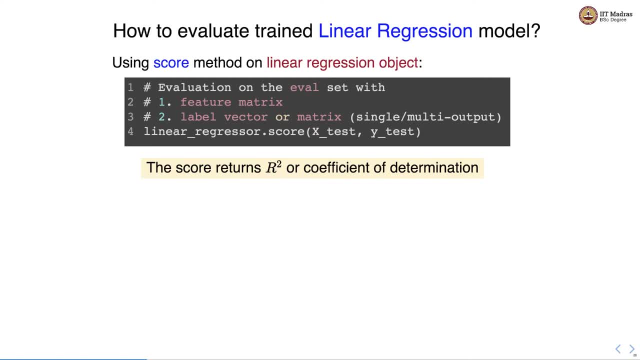 a quantity which is known as R square or coefficient of determination. Let's see what this R square is. Let's see how this R square is computed. So R square is computed as 1 minus u by V, where u is residual sum of squares and this 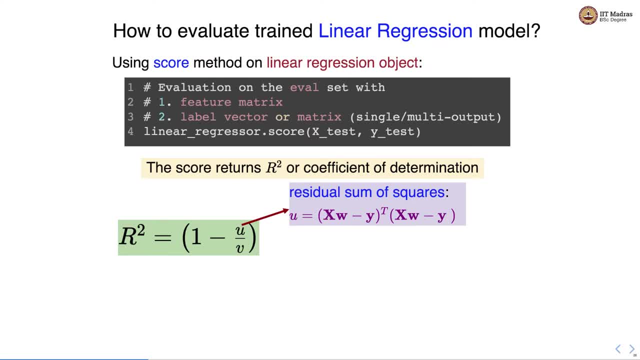 is a familiar equation to us: XW gives us the predicted labels, Y is actual label, and this is nothing but the difference between the predicted label and actual label. So XW is the actual label, XW is the actual label. This is the actual label. This is the actual label. This is the. 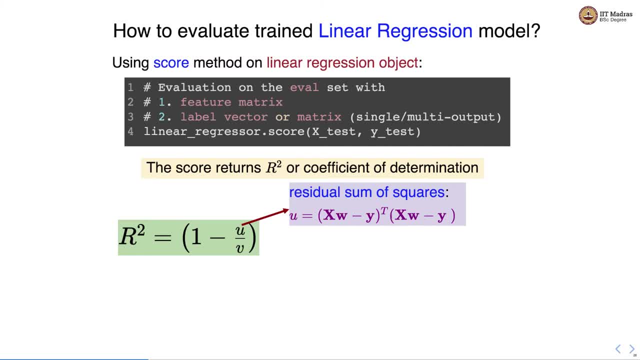 actual label. We take the transpose of this different set and multiply it with itself. So this is like finding the square of difference between the predicted labels and actual labels. which is what is the loss function for the linear regression? On the other hand, v is: 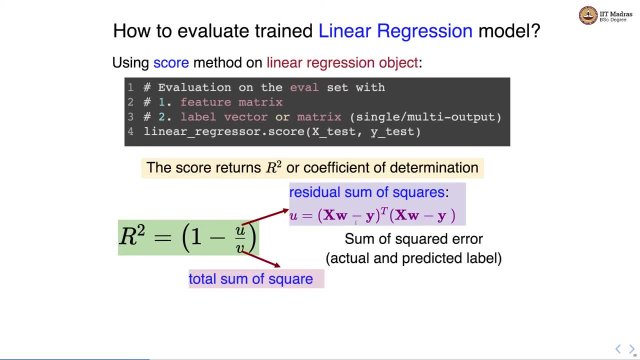 total sum of square, and this v is computed as a difference between the actual label minus the mean of the predicted label. We take, transpose and multiply this difference vector with itself. So this is square of difference between the actual label and the mean of the predicted. 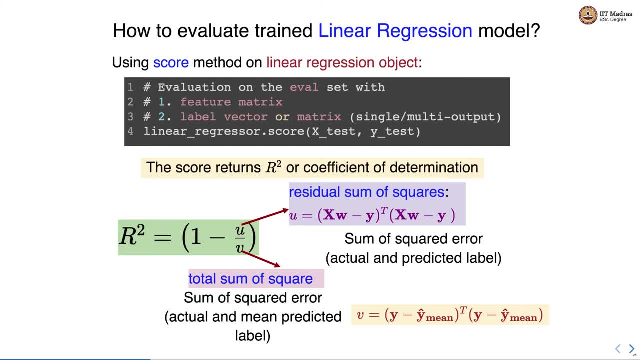 label. So here it was a predicted label, but here we take mean of the predicted label and that's how we calculate what is called as sum of squared errors. So now this is also sum of squared error, but this is sum of squared error between actual and mean predicted label. 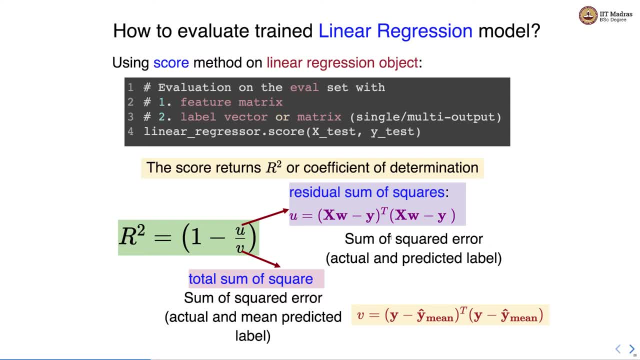 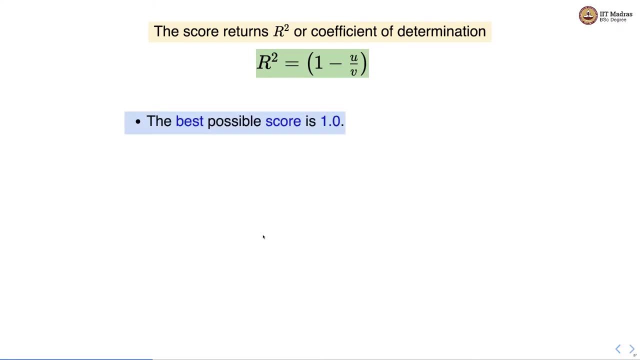 whereas u is sum of squared label, sum of squared error between actual and the predicted label. So r square has the best possible score of 1.. A constant model that always predicts the expected value of y would get score of 0. And the score can be negative because model. 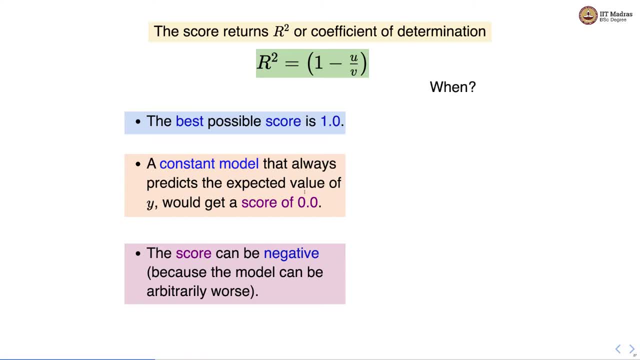 can be arbitrarily worse. Let us see when these scores occur. So we get score of 1, when u, that is, the sum of squared error between actual and the predicted label, is equal to of squared error is zero. so when u is zero, obviously this quantity is zero. so one minus. 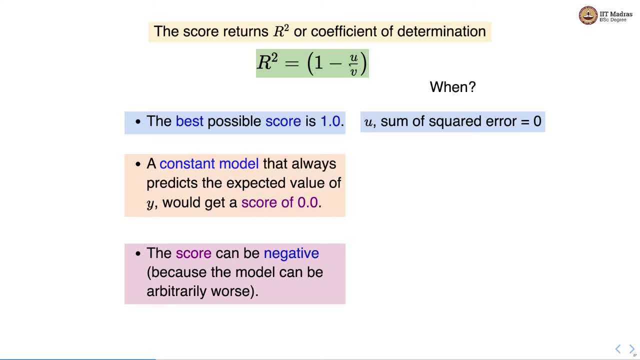 zero is one, so we get r square of one. when u is equal to zero, a constant model that predicts the expected value of y would get score of zero, and that would happen when u is exactly like v. this is the total sum of squared error and this is the residual sum of squared error. 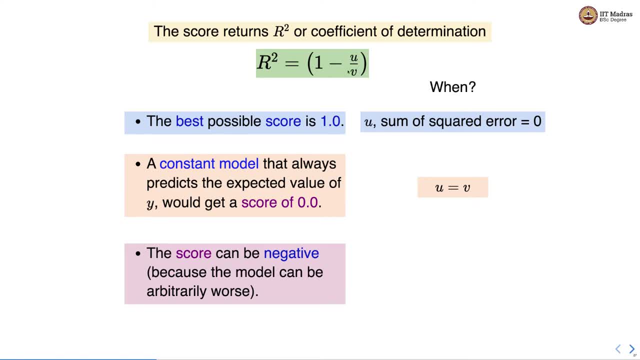 for this we calculate. this particular quantity is calculated as the difference between the actual label minus mean of the predicted labels, and this quantity is calculated as the difference between the predicted label and actual label. and then we square it up, so when the predicted label is exactly equal to the mean of all predicted labels, we will get into a situation: 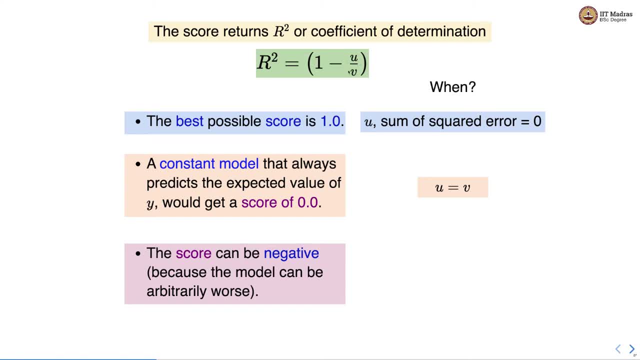 where you will be exactly equal to v, and when that happens this quantity becomes one, and one minus one becomes zero. so r square returns the value of zero, and if model is arbitrarily worse, u is expected to be greater than v, and then the score can become negative. so, apart from 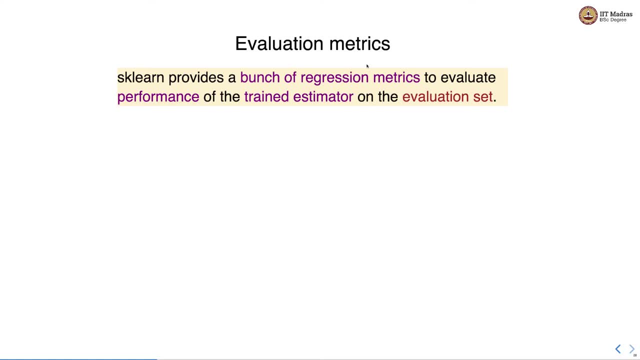 score. so score method returns r square. but there could be other regression metrics that could be of our interest. fortunately, sklearn provides a bunch of such regression metrics for us to evaluate performance of the trend estimator on the evaluation set. let's look at those evaluation metrics. the first one is mean absolute error. so all these metrics? 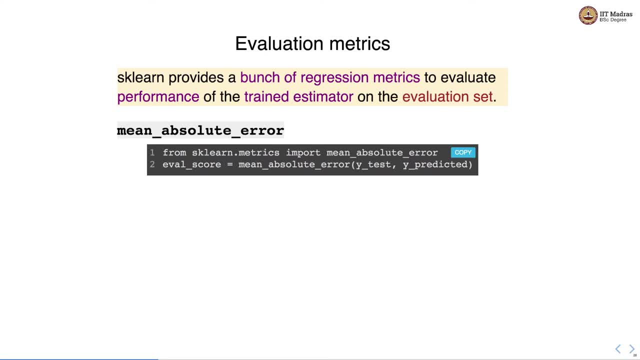 are implemented as part of sklearn dot metrics module. we can. we can import these, these metrics, one by one. so from sklearn dot metrics import mean absolute error and we calculate mean absolute error by supplying the actual labels and the predicted labels. so this particular, this particular function would return the score, that is mean absolute error minus the. 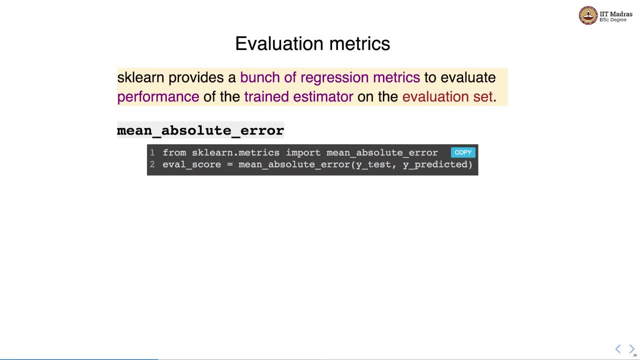 actual values, between the predicted values, between the predicted values and the actual values. in the similar manner, we have mean squared error, which is which is again implemented as part of sklearn dot metrics package, and we can we calculate this mean squared error exactly like mean absolute error, where we supply the actual labels and the predicted. 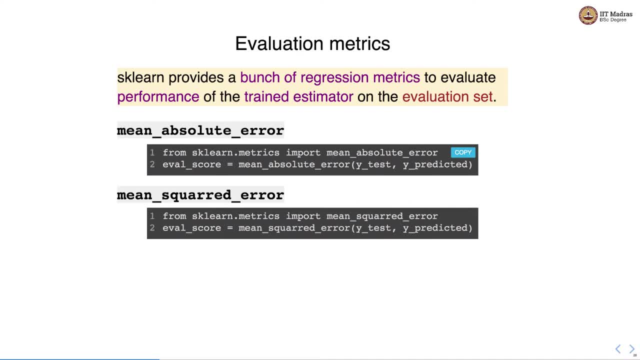 labels. so you can see that all these, all these metrics need two argument: one is the actual label and second is the predicted label, and then that particular metric is applied on this, on the supplied arguments, and we get the evaluation score. then there is r2 score, which gives same output as the score method. 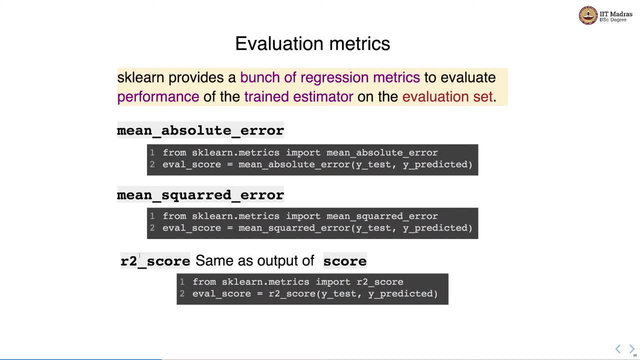 and this r2 is exactly what we saw in the previous slide, which is the coefficient of determination. so we we import r2 underscore score from sklearn dot metric module and we supply the actual values and the predicted values to obtain the r2 score. so all these metrics can also 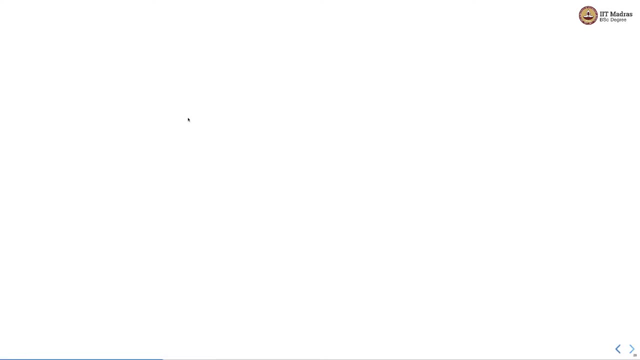 be used in multi output regression setup. then we have additional metrics that that are not amenable to multi output regression setup. we can also use multi output regression setup. so one is mean squared log error and this particular metric is useful for targets with exponential growth. so when our labels denote exponential growths, like population sales, 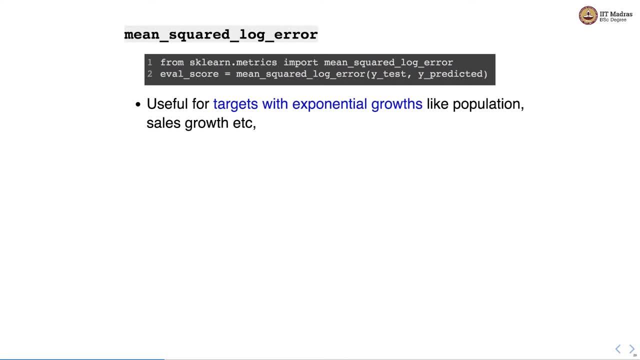 growth of a company, etc. then we use mean squared log error. so this particular metric penalizes underestimation heavier than the overestimation. then we have mean absolute percentage error, which is sensitive to relative error. so when we want to evaluate our predictions that are sensitive to relative errors, we should be using mean absolute percentage error. 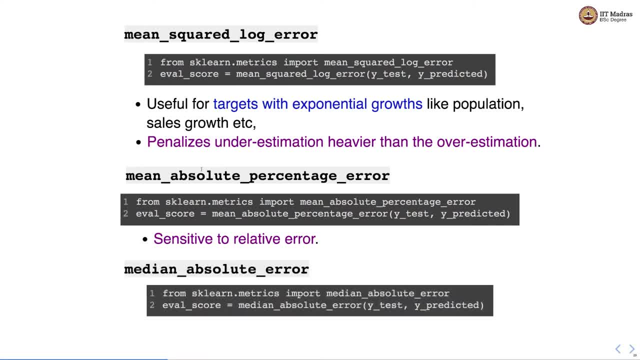 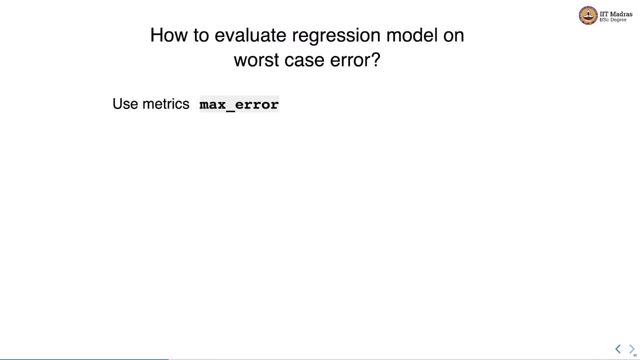 we also have mean absolute error, which is robust to outliers. it doesnt give a lot of importance to the outliers and our our evaluation becomes robust to the outliers. so let's see how this work out. 1.. 1. how to evaluate regression model on worst case error. So we can use metric max underscore. 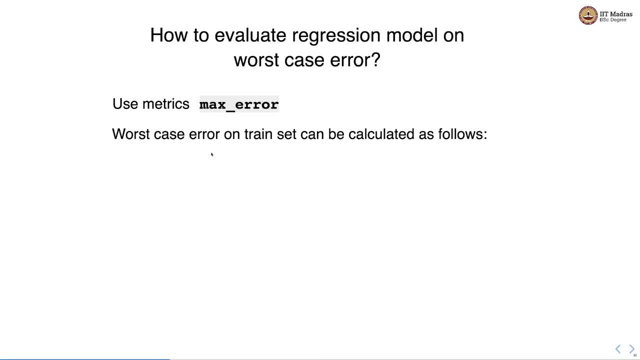 error which gets us worst case error. Let's first calculate worst case error on training set. So we import max underscore error from sklearnmetrics and we supply the actual values and the predicted values. In this case we supply the training labels and the predicted training labels and we calculate the worst case training error, The worst case error. 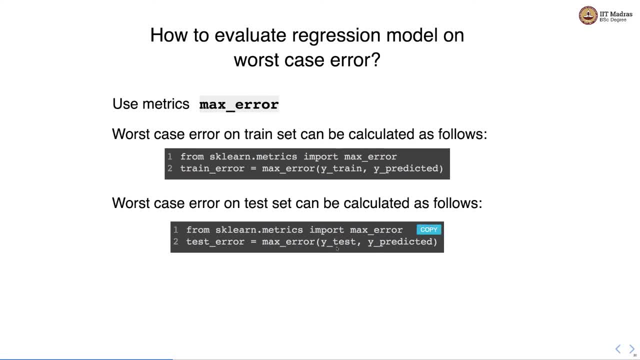 on test data can also be calculated in a similar manner where we supply- instead of training, we have supplied test labels and the predicted test labels to get the worst case error on the test set. This metric can only be used in single output regression. It does not support. 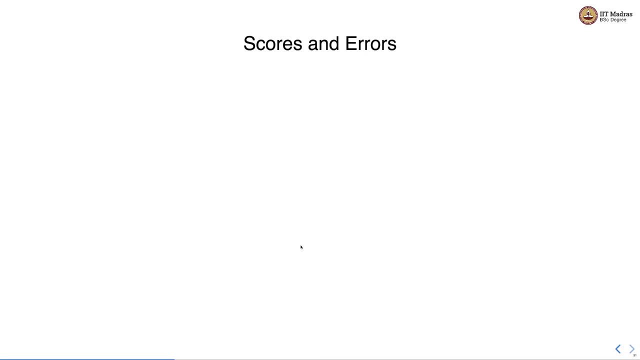 multi output regression. So, while studying these metrics, you will come across two terms: the ones that are ending in scores and the other metrics that are ending in errors. So score is a metrics for which higher value is better, and error is a metric for which lower value is better. So let's 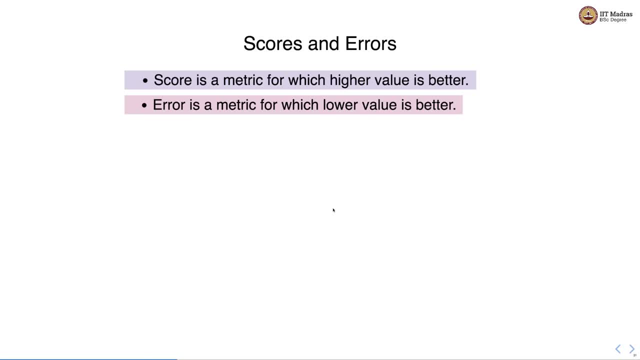 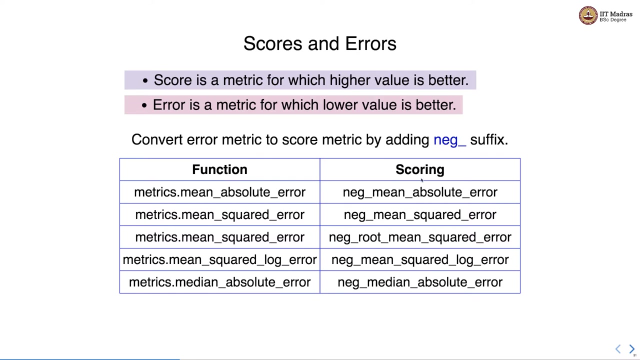 keep this convention in mind while evaluating regression models or, for that matter, any other estimator in any other estimator class. So we convert error metric to score metric by adding neg underscore suffix, For example. these are some of the error functions that are there in sklearn and on the right hand. 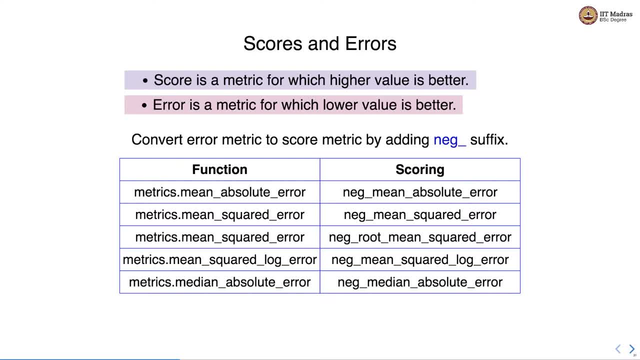 side we see the corresponding scoring functions. For example, mean absolute error. is the error function or is the error metric that is defined in sklearnmetrics? The corresponding scoring function is neg underscore- mean absolute error. So you can see that we have added a neg underscore suffix to this particular error metric and we got this particular. 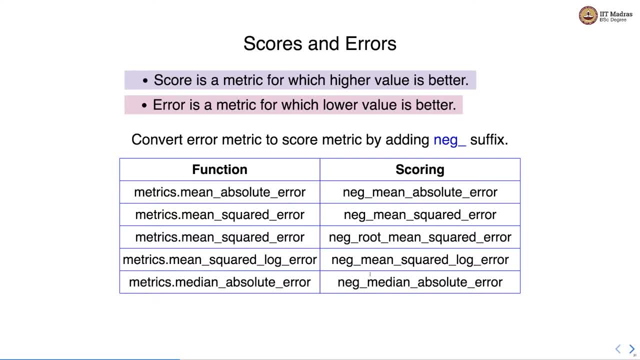 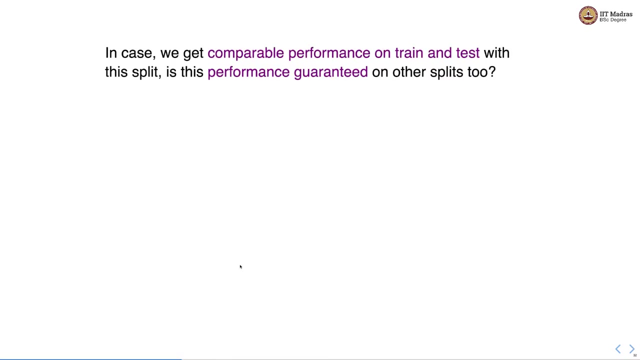 scoring metric And you can see that pattern getting repeated throughout this table. So for mean underscore, square underscore error, the corresponding scoring metric is neg underscore, mean underscore, square underscore error. Then we have similar scoring, corresponding scoring metric for mean square error, mean square log error and median absolute error. 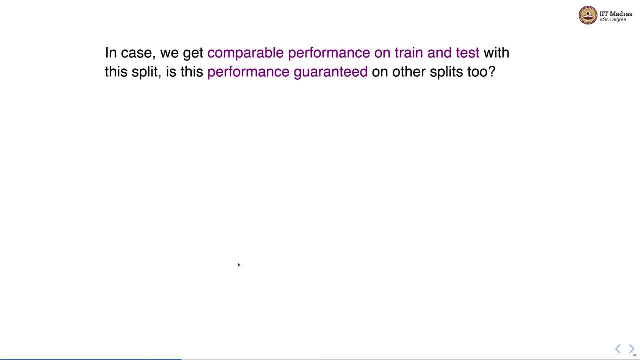 So now in case, when we get comparable performance on training and test set with a particular split, is this performance guaranteed on other splits? So you remember right, I mean we use train underscore, test underscore split function to get a split on training and test set. that 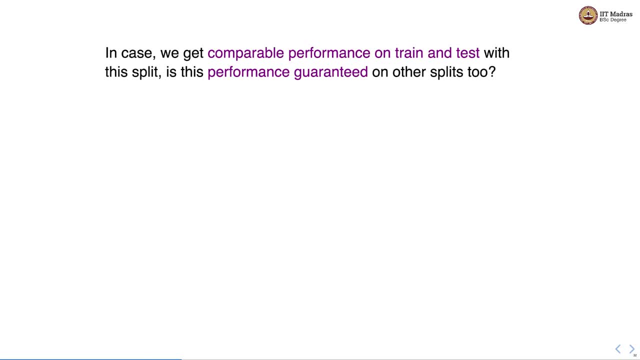 was a single split that we got. So what is the guarantee that the performance that we have gotten on this training and test split is also replicable or is also guaranteed on other splits? So there are a couple of questions. Is the test set sufficiently large In case the test 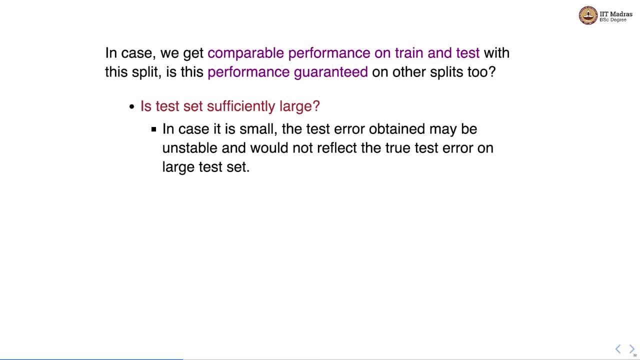 set is small, the test error obtained may be unstable And it would not reflect the true test error on the larger test set. Second question is: what is the chance that the easiest examples were kept aside as test And if this happens we would get optimistic estimation of true test error And both of 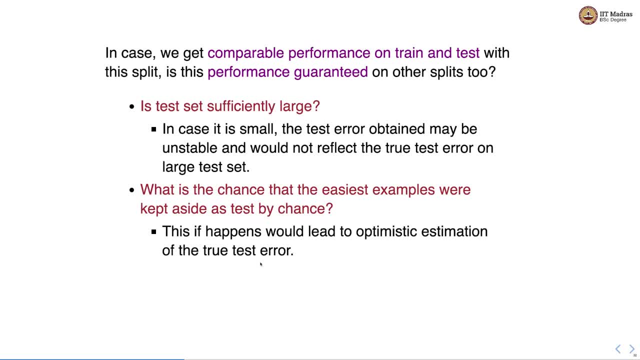 the situations are not really good as far as evaluating the generalization of the test, So we will have to wait and see. So what is the chance that the test will give us the correct estimation of the generalization error or the test error of the model? And they will not give us the right kind of estimate. 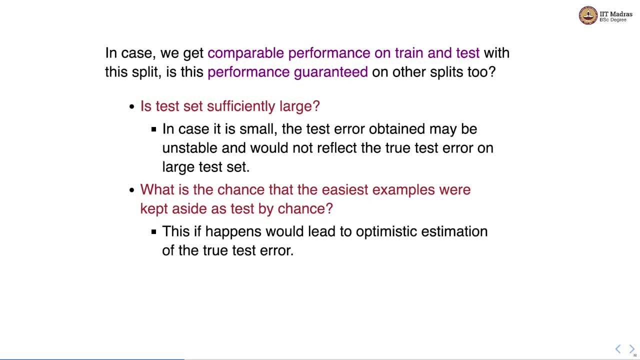 about how model will perform on unseen data when deployed. So we knew we need something better And fortunately we have a cross validation tool. We have studied cross validation in detail in machine learning techniques class and here we'll use this cross validation. So cross validation: what it does is it creates. 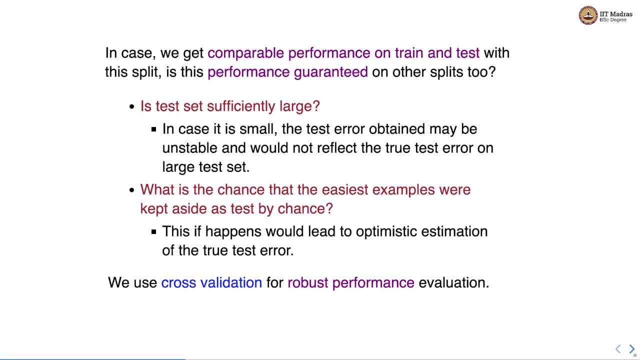 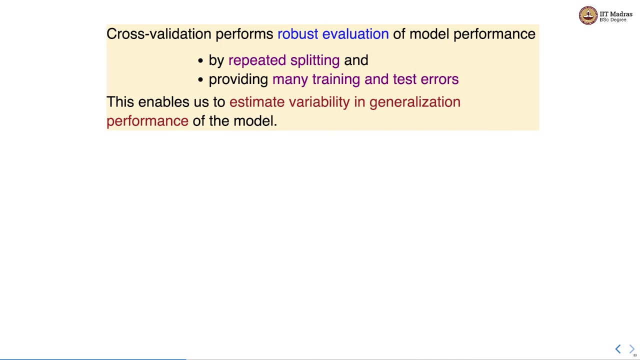 multiple training and test sets and it evaluates the performance on different test set. That way we are using different test splits and hopefully, when we perform this evaluation of multiple test splits, we get robust performance evaluation. So cross validation performs robust evaluation of model performance by repeated splitting. 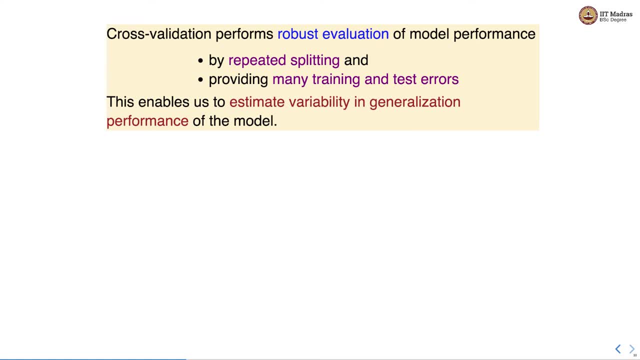 and providing many training and test errors. This enables us to estimate variability in generalization performance of the model. So sklearn implements the following cross validation iterators: So we need to know how to perform these splits and there are various ways in which these splits are performed. 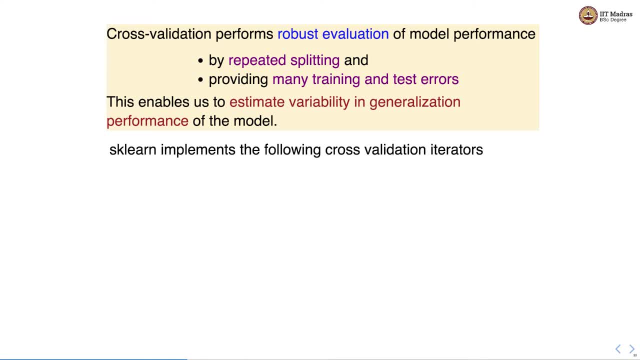 These splits can be made and sklearn implements different cross validation iterators. So there is this k-fold cross validation iterator, which is very similar to what we have studied in machine learning techniques course, where we divide data into k different folds or k different partitions, and then we select k minus 1 partitions for training and 1 partition. 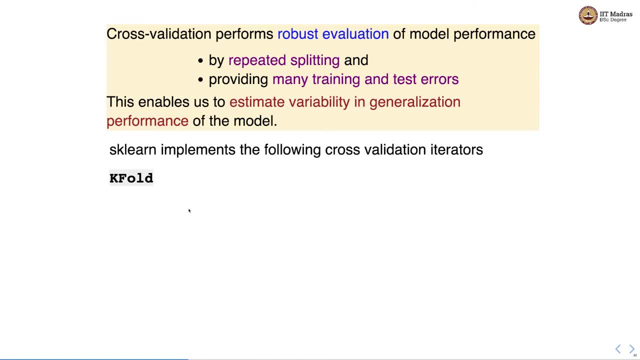 for test or for evaluation, And we do this for for different splits of these k partitions. That way we get multiple training sets as well as evaluation sets. Then we have another iterator called as repeated k-fold. this essentially repeats the k-fold splitting. Then we have leave1 out, which is 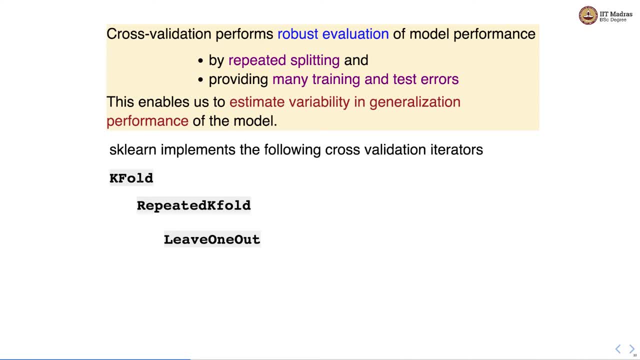 a special case of k-fold where k is equal to number of training samples. So in leave and out we leave out exactly one example as a test and we use rest n minus 1 examples for training. So we get n such different splits on which we can perform training, as well as the evaluation. 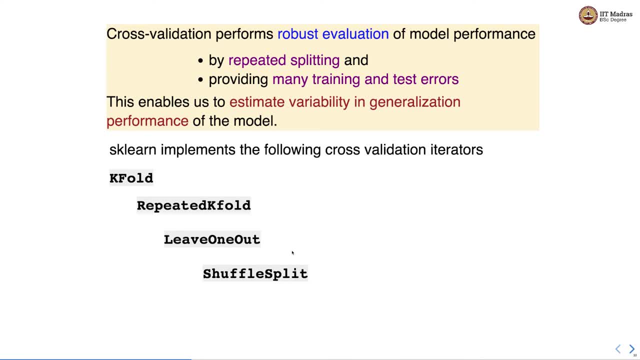 And finally, we have shuffle split, which shuffles the training data before splitting and it ran and it does a random permutation of the data points and create training and test sets And it does it repetitively for a specific number of times that is specified by the user. 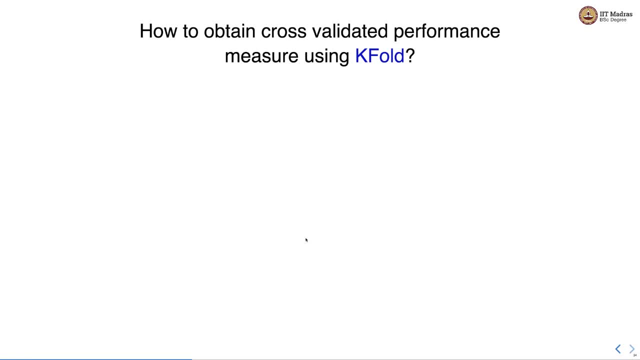 So let us try to find out how to align, obtain cross-validated performance measure using k-fold. So here we use a cross underscore val underscore score API implemented in sklearn dot model selection module. So we have linear regression estimator. and on this linear regression estimator we want 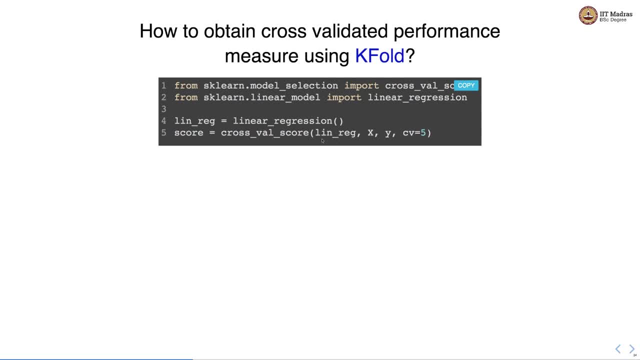 to calculate cross-validation score. So we provide the name of the estimator, the feature matrix, the label, the label vector or label matrix, depending on what kind of regression problem we are solving, and we also specify number of folds in cross-validation. When we specify an integer value to the CV parameter of cross-validation score, it uses. 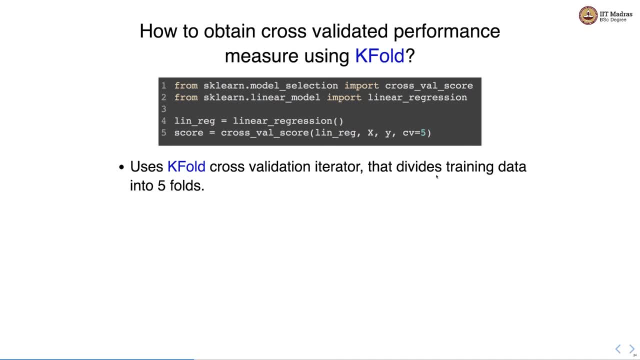 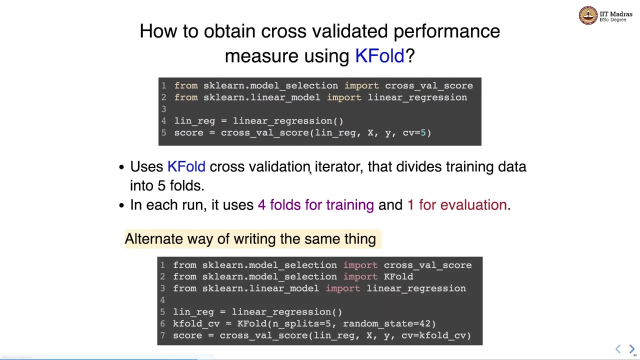 k-fold cross-validation iterator and divides the training data into the specified number of folds. It uses four folds for training and one fold for evaluation. This is an alternate way of writing the same thing, where we will explicitly be using k-fold- k-fold cross-validation iterator. 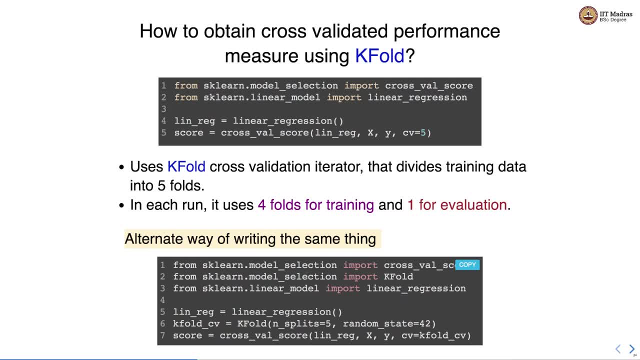 So we import k-fold from sklearn dot model underscore selection module and we instantiate an object of a cross-validation- 1. k-fold iterator, by specifying number of splits and a random seed. Then in cross validation score, instead of specifying an integer value over here, we specify: 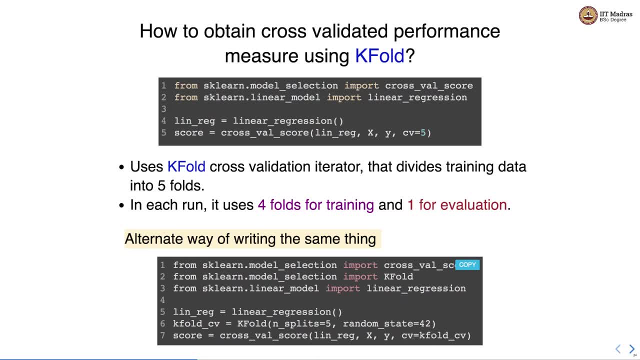 the k-fold object and when we specify this k-fold object, it performs the k-fold. it actually does the cross validation with k-fold iterator. So these two code snippets exactly do the same thing. In case we want to use different cross validation iterator, we can simply choose one from the 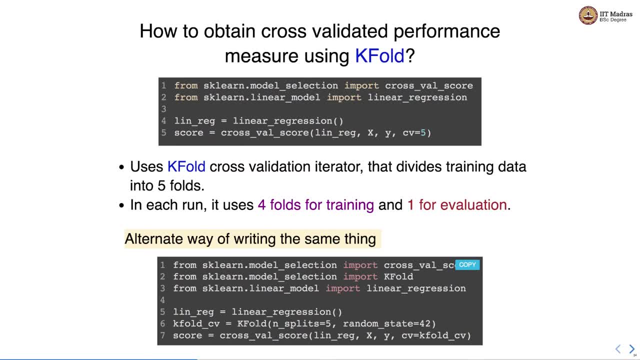 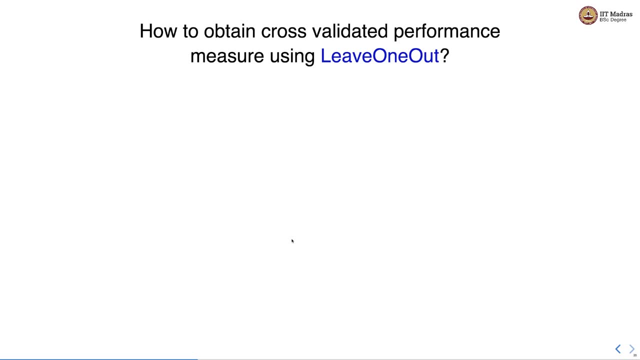 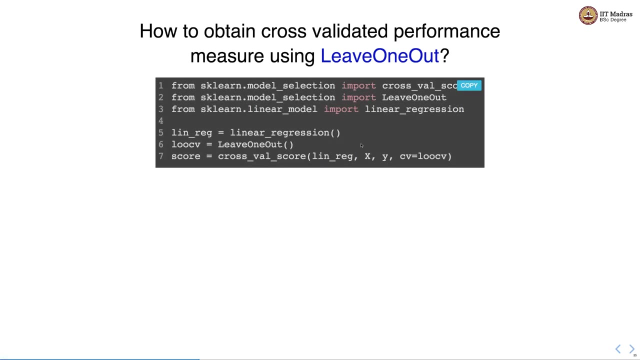 model underscore selection module, instantiate that object and specify that cross validation iterator in the cv parameter of cross validation score. Let's see couple of examples of that. Let's first see how to use leave an out- Leave an out cross validation iterator for calculating the cross validator performance. 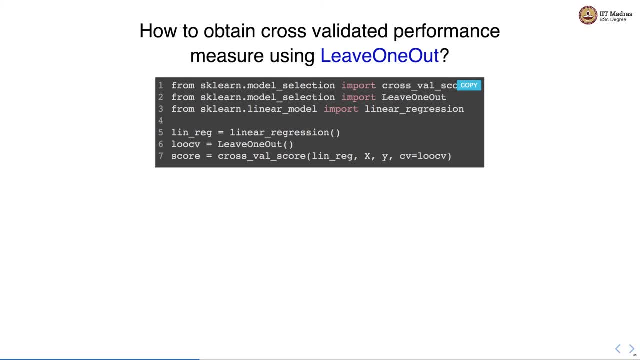 So here we import, leave one out, class from sklearnmodel underscore selection module. So you can see that all model underscore, all model selection related utilities are presented, are present in model underscore selection module of sklearn, and this is because of the design principles of sklearn API that we studied in the first week of machine learning. 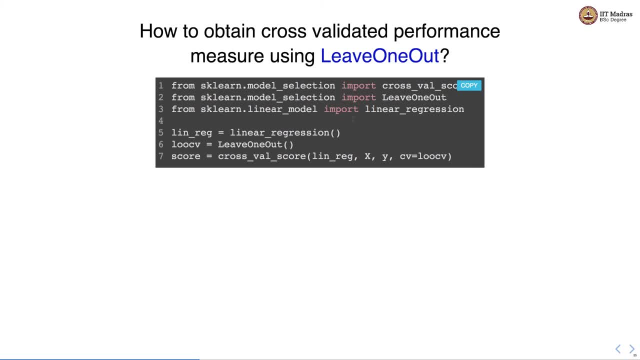 practice course. So here what we do is we instantiate an object of leave one out cross validation iterator and that object is used as a parameter for the cv parameter. That object is used as a value of cv parameter in cross validation score. So when we do that, 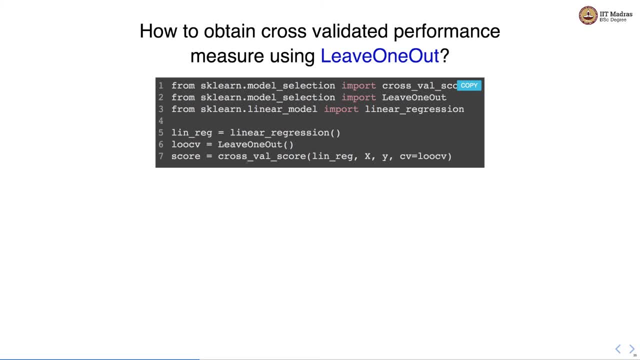 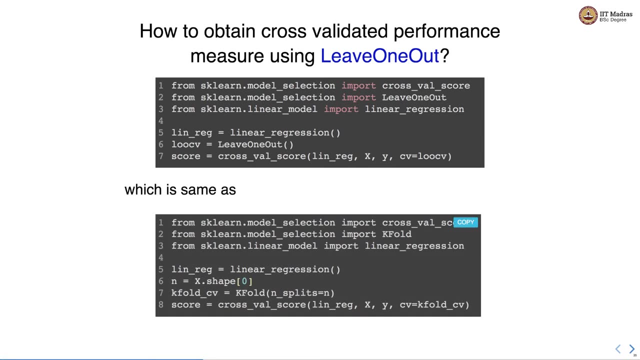 So when we write this particular, when we execute this particular statement, we get a score that is calculated using- leave one out- cross validation iterator. Now, this is same as using k-fold, using k-fold cross validation with number of splits equal to n, which is, which is essentially the number of samples in the in the training set. 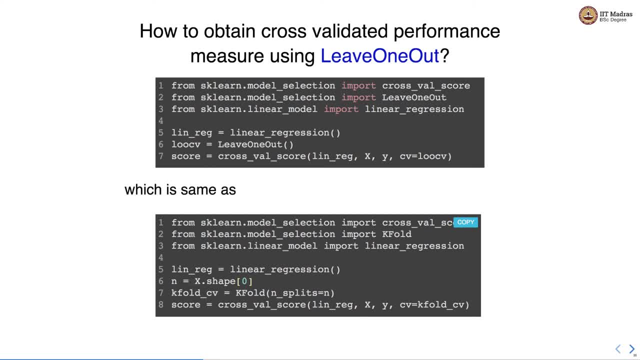 So here what we do is we first calculate the number of samples in the training set and we set n splits to n in k-fold cross validation and then we calculate the cross validation score with the, with the object of k-fold, k-fold cross validation iterator as a value. 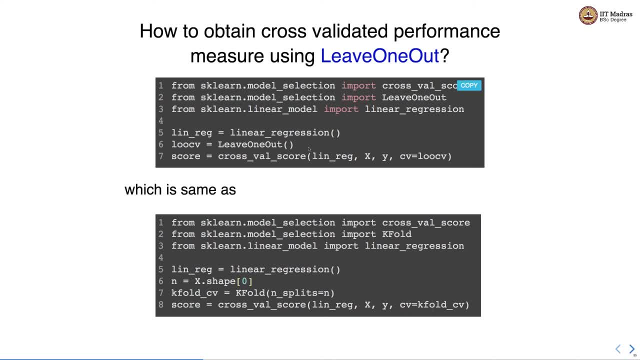 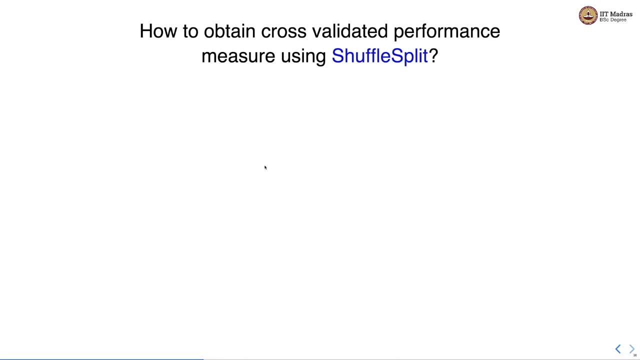 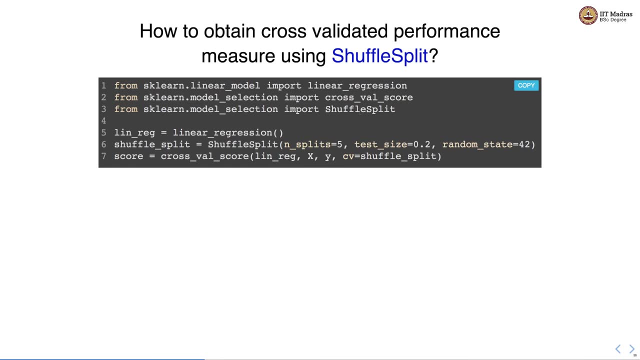 of cv parameter. Again, these two code snippets would do the same thing. Let's look at how to obtain cross validated performance. Let's see using shuffle split. Again, the strategy is the same. we import shuffle split, we instantiate object of a shuffle split by specifying number of splits, the size of 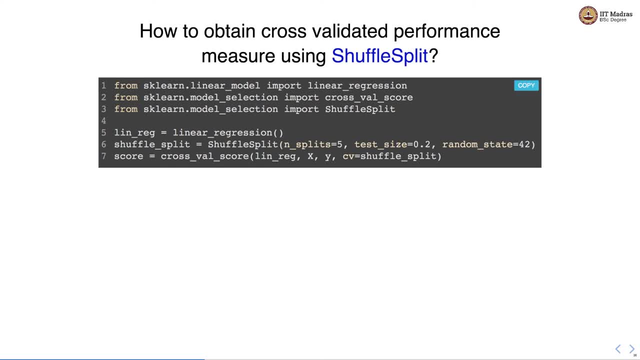 the test and the random seed, and we use that shuffle split object as the value of the cross validation parameter in cross validation score function. Shuffle split is also called as random permutation. It generates user-defined number of trained test split as specified in n underscore splits, and it 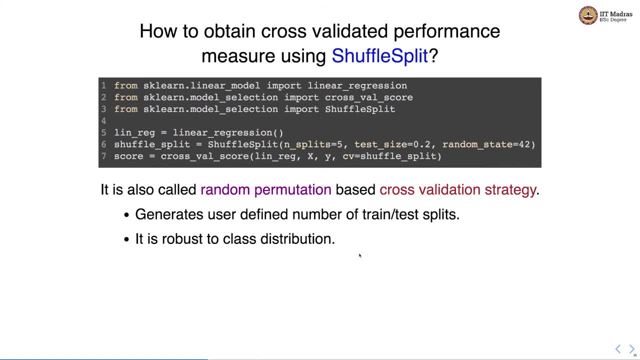 is robust to the class distribution. So even if there are different class distributions, if we do not have uniform class distribution, even in that case shuffle splits work. We have developed it reasonably well In each iteration. shuffle split shuffles order of data samples and then splits it into training and test. 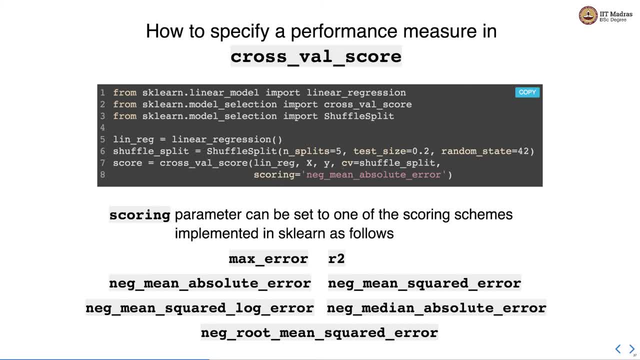 So far we were using a default scoring mechanism for calculating cross validation score. Now, here we will try to specify the default score for the given data sample. Now here we will try to specify the scoring mechanisms. So we have already seen some of the scoring metrics which correspond. 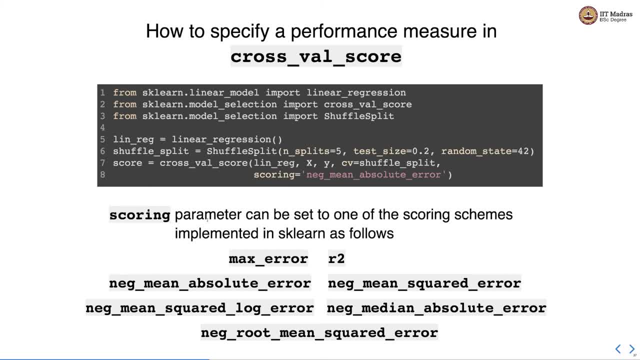 to error metrics before few slides. So scoring parameter can be set to one of the scoring schemes implemented in sklearn. So we can use max error, R2 or all these negative of the error metrics that is: negative mean absolute error, negative mean squared error, negative. 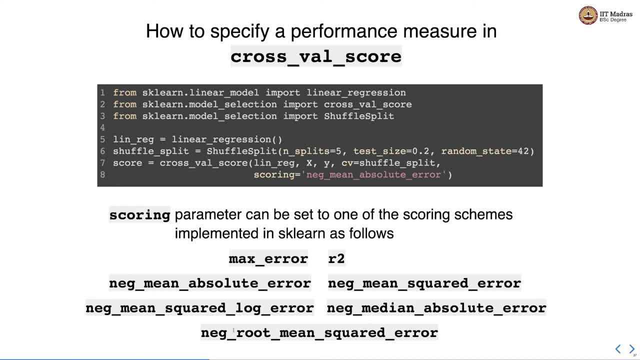 mean squared log error. negative median absolute error and negative root mean squared error. So we can substitute these values in the scoring parameter and we get that particular score by after doing the cross validation. So since we are doing cross validation, hopefully these scores are robust than calculating these scores. 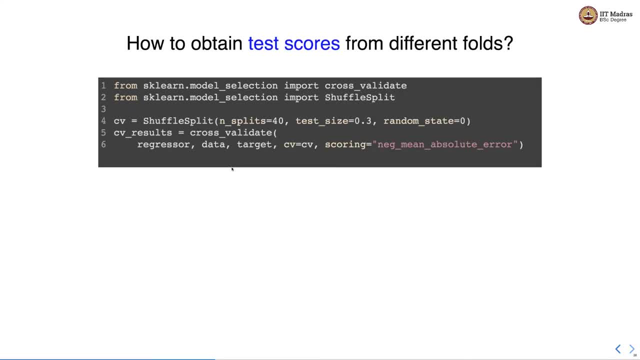 scores just on a single training and test split. Let's see how to obtain test scores for different folds. So here, what we have done is we have used shuffle split cross validation iterator with number of splits to be 40, size of the test is 30% and random seed equal to 0.. 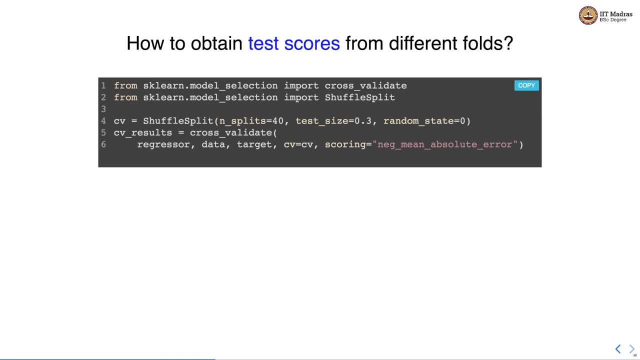 Then we calculate, then we call a cross validate function. So instead of calling cross val score, we are now calling cross validate function with parameters. which is the estimator, which is the regressor, the data, which is the feature matrix. target is the label, label vector or matrix, depending on whether we are solving. 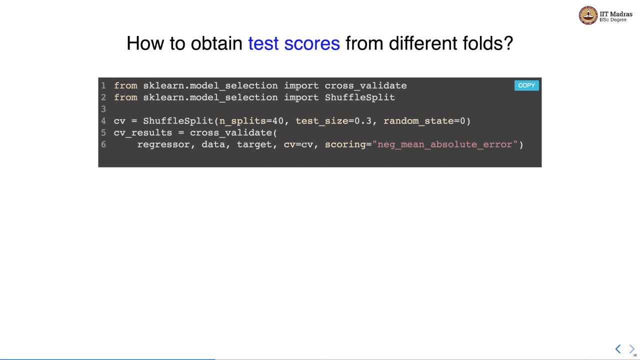 single or multi-output regression problem, Then the cross validation iterator And we also specify the scoring scheme. Now this cross validate returns returns this result, which is essentially a Python dictionary, with the following keys: It has got fit: time score, time test score estimator and train score. 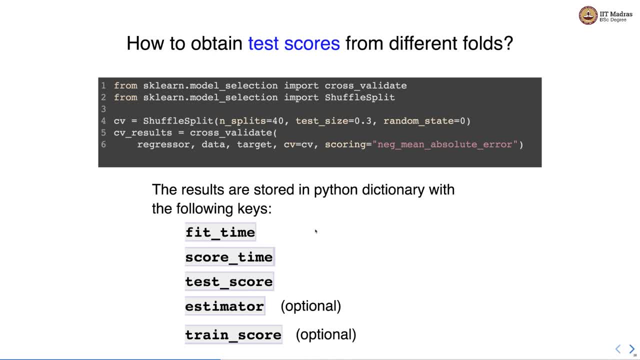 Estimator and train score are optional and in order to obtain them we need to specify additional parameter To cross validate. by default we do not get estimator and train underscore score, So fit underscore time gives the time that was required for fitting that particular training. 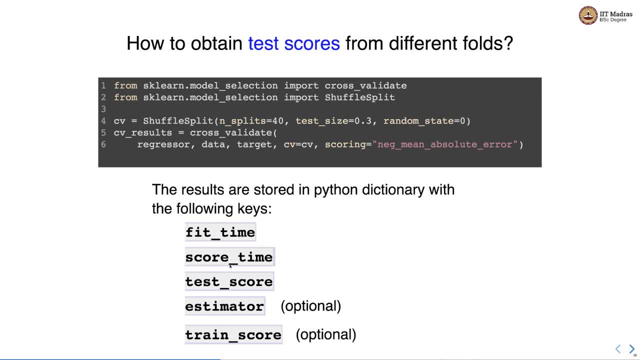 for fitting the regression model on that training set. Score time is the time it took to get the score on the evaluation set, and test score is actually the score that was obtained on the evaluation set. So fit underscore time gives the time that was required for fitting the regression model. 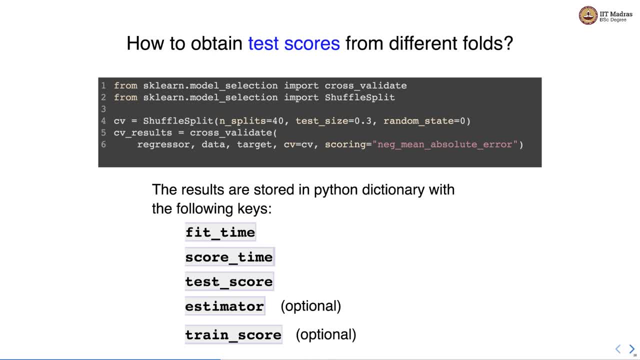 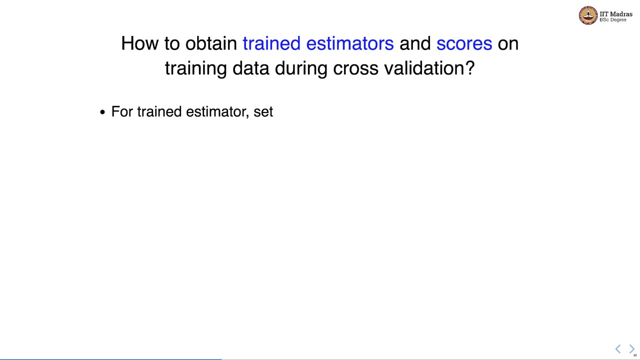 on the evaluation set And the score in this case would be negative, mean absolute error, because that is what we have specified in the scoring parameter. In the same manner, we can also obtain trained estimators and scores for each fold. For obtaining trained estimator, we need to set return underscore estimator parameter. 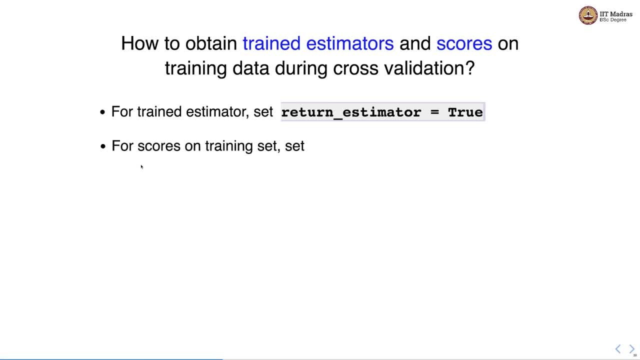 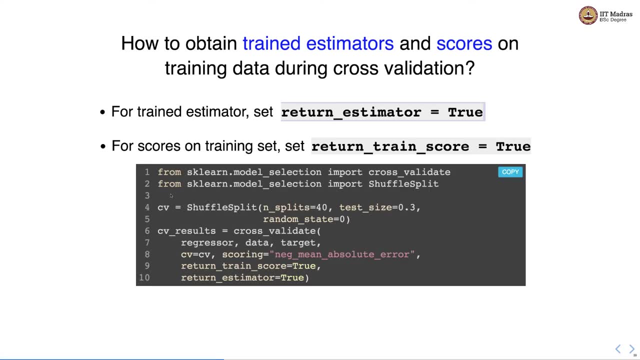 to true. It is false by default. For scores on the training set, we need to set return underscore estimator to true. For scores on the training set, we need to set return underscore estimator parameter to true. Let us look at an example. 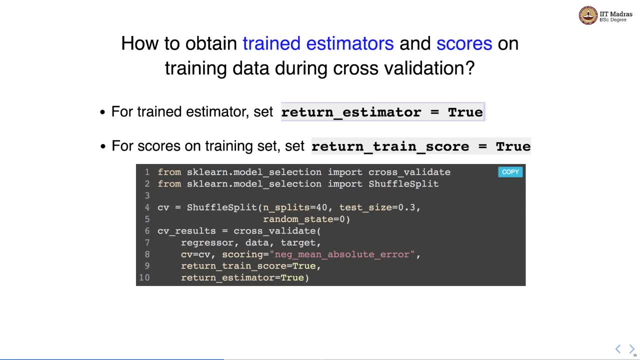 So here we are calling the cross validate function by specifying all those parameters that we saw in the previous slide. In addition to that, we are specifying couple of more parameters, which is return underscore, train underscore score, setting it to true and return underscore, estimator and also setting. 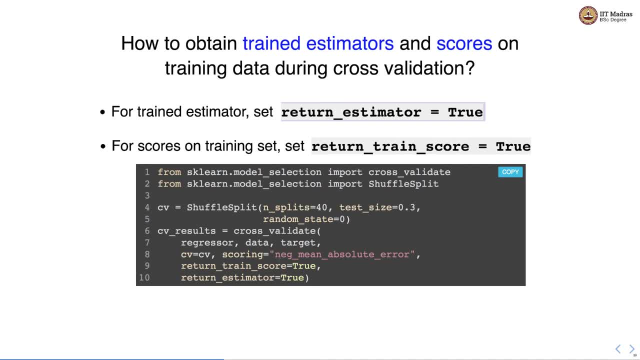 that to true. When we do this, we get in this particular dictionary, which is cv underscore result. we get different estimators that were trained on different splits. We also get the training scores. That helps us to compare training and test scores as well as we can. we can also examine 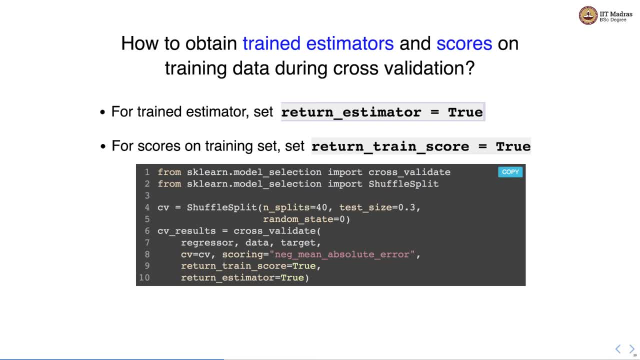 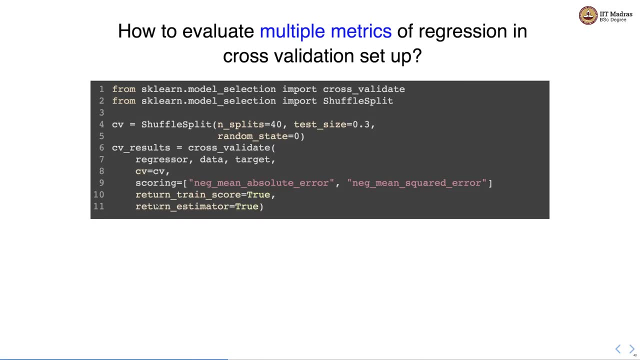 these estimators that were run, that were learned on different splits. The estimators can be accessed to estimator key of this dictionary: So cross validate. so cross validate function also allows us to specify multiple scoring matrix. This facility is not available in cross validation score function. 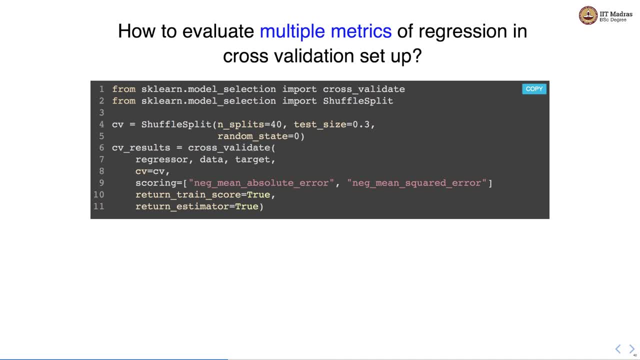 So that is the main difference between cross validate and cross validation score. Cross validation score also only returns the score on that only returns the score after cross validation, Whereas cross validate returns- It returns a lot more information, like it returns the score for every fold. 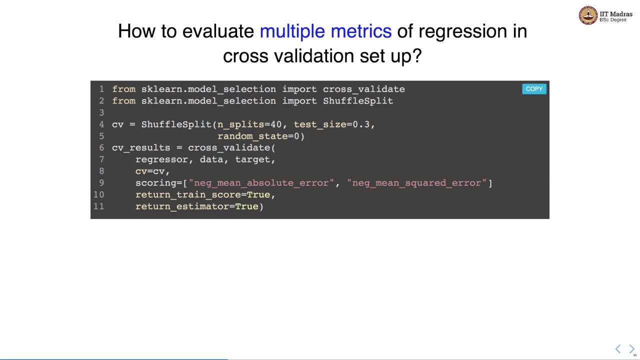 It also returns the estimator and the training error that was. that was, that it obtains on different folds while performing cross validation. So in this case we have specified couple of scoring parameters. One is negative mean absolute error and negative mean squared error. 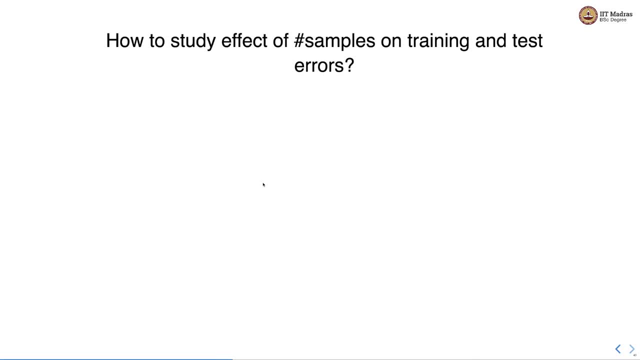 So let's see how to study effect of number of samples on training and test errors. So sklearns provide us. sklearn provides us with learning underscore curve class. This learning underscore curve class takes estimator training data, size of the of the training, cross validation strategy and score. 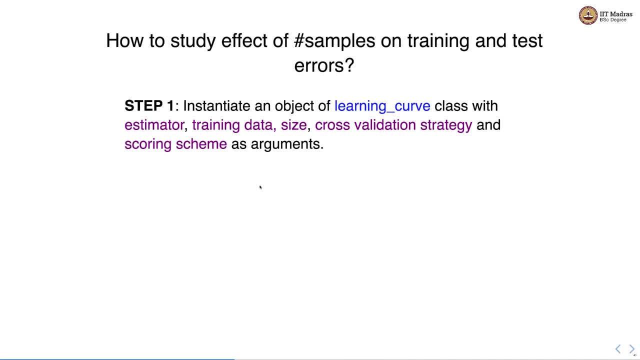 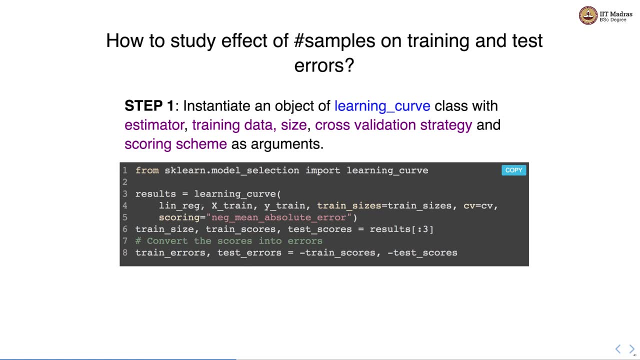 Scoring scheme as arguments, which is pretty much same as the cross validate function. So we instantiate an object of learning curve by specifying the linear regression estimator, training training, feature matrix, label matrix, the size of the training training data. then 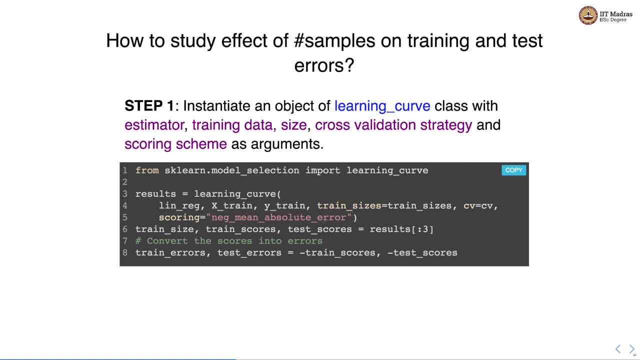 the cross validation iterator and the scoring scheme And we can get the training size. We can get the training score and test score by by accessing first three values of of this particular results that was written by learning underscore curve. We can convert. since these are scoring schemes, in this scoring we are using basically the 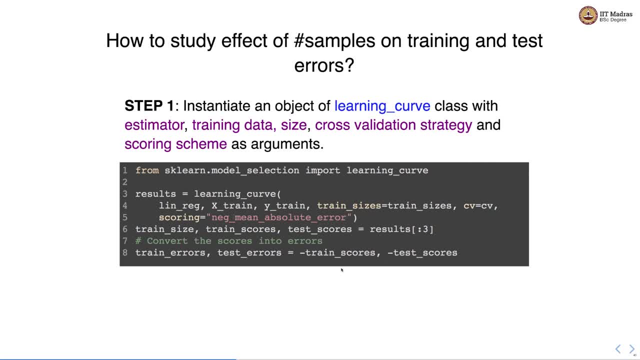 the negative error. So, in order to obtain the actual errors, we multiply each of these scores by minus one. So we multiply the train score by minus one, We get train error. We we multiply test score by minus one, We get test error. 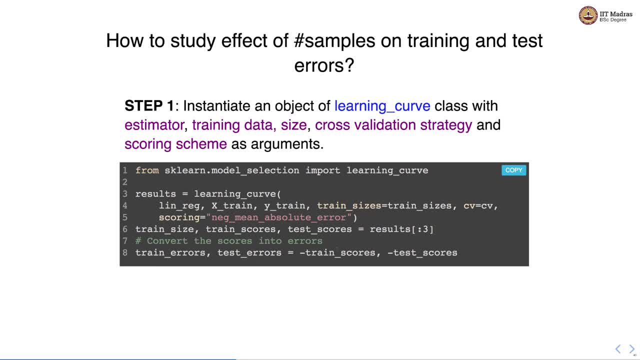 This is how you can convert scores into errors. if you want to output the error due to due to a specific training or specific evaluation set for that estimator. In step two, we generally plot training and test scores as function of the size of the 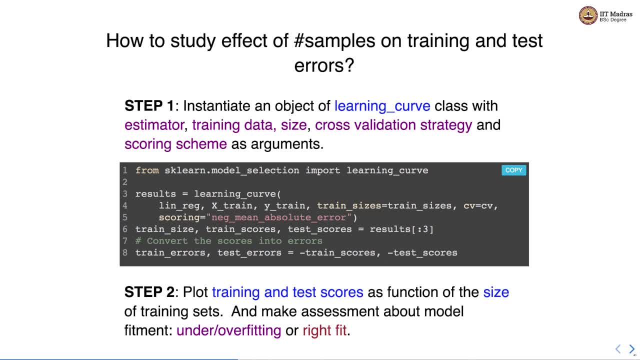 the size of the training set, And this plot helps us to make assessment about the model fitment. We can. we can diagnose whether model is model is just a right fit or whether it is underfitting or overfitting, and then take appropriate measures to alleviate any of such.